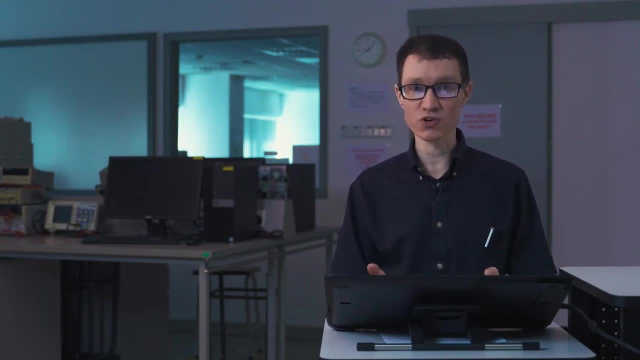 wait long enough. then, no matter how big the inductor is or no matter what its inductance is, the current flowing through the capacitor will keep flowing. that inductor will be the maximum amount of current that the battery can give you. Let's take a look at a few examples now. 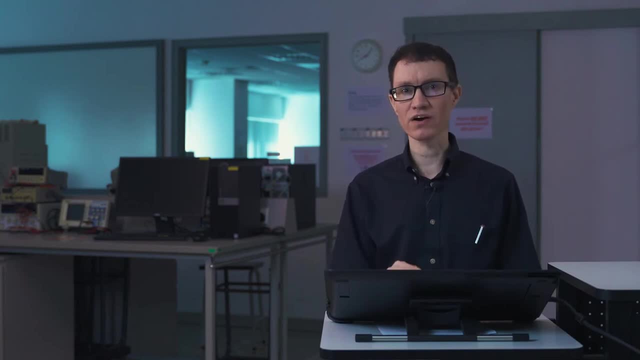 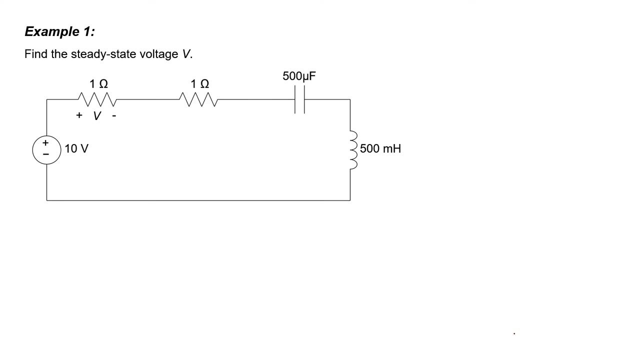 of inductors and capacitors used in circuits where this information can be useful In this problem. we're told to find the steady state voltage V across that resistor. We see capacitors and inductors in this circuit And one way to approach the problem. 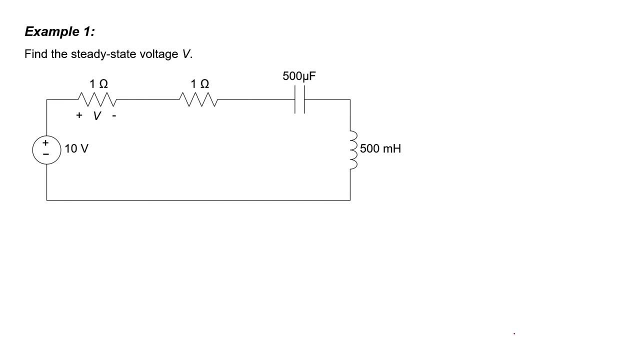 would be to start writing down differential equations, But we can use some important information about capacitors in order to make this problem incredibly easy. We know that, initially, if the capacitor is not charged, then current will have to flow from the 10-volt source. 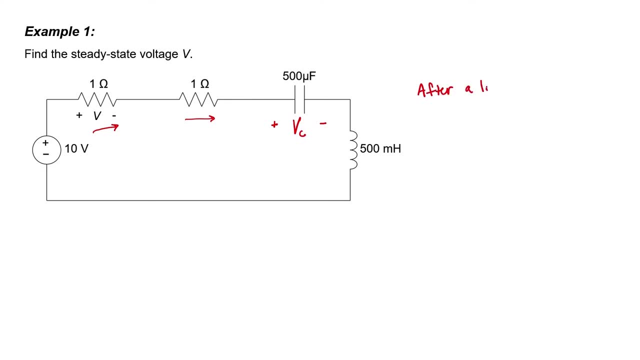 over into the capacitor. Eventually, that 500-microfarad capacitor will be charged to 10 volts. In this problem, that's what the words steady state mean. What happens after a long period of time If we know that this voltage is eventually? 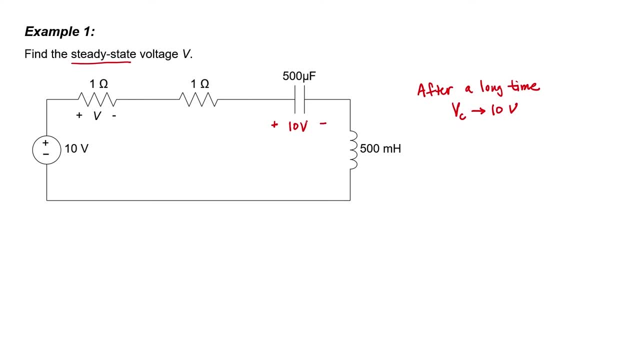 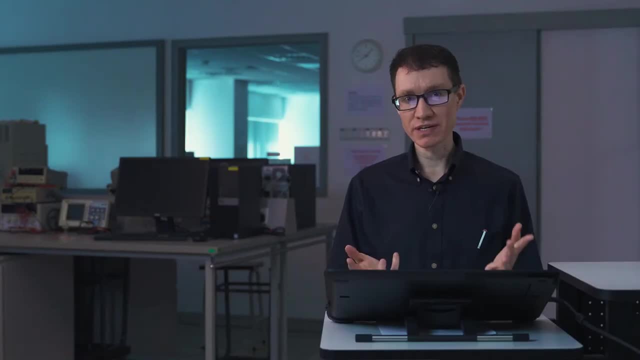 going to be 10 volts. At that point, current will stop flowing. Let me redraw the circuit to make it clear. The amount of time it takes for that capacitor to reach 10 volts of course depends on the value of the other components in the circuit. 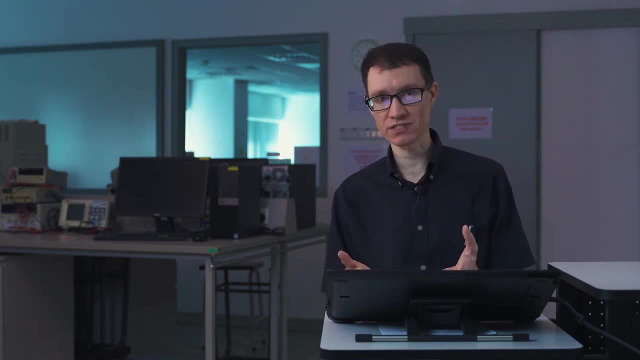 If you use larger resistors, it takes longer for the capacitor to charge. If you use a larger inductor, it takes longer for the current to get flowing through that inductor in order to get the capacitor charged up. But if you wait long enough then eventually. 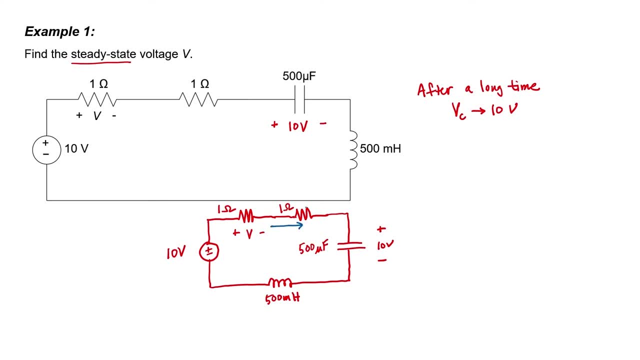 that capacitor is going to be charged to 10 volts And when that happens, the current flowing through the two resistors is going to be 0. And the current flowing through that inductor is also going to be 0.. Using Ohm's law, I know that V equals IR. 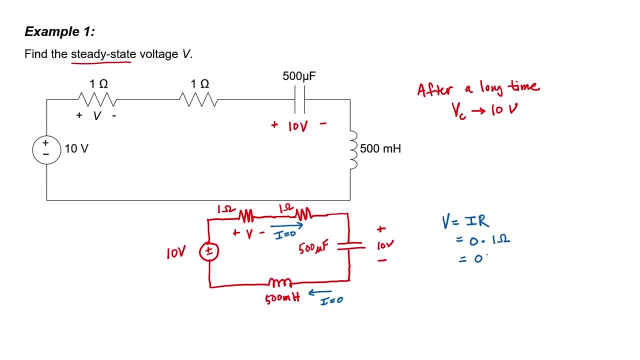 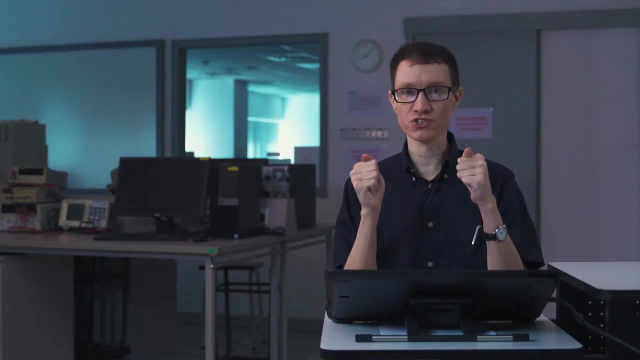 The current is 0.. The resistance is 1 ohm, Therefore the voltage is 0.. In steady state or after a long period of time, no current flows through that resistor. Therefore the voltage drop across it is 0.. 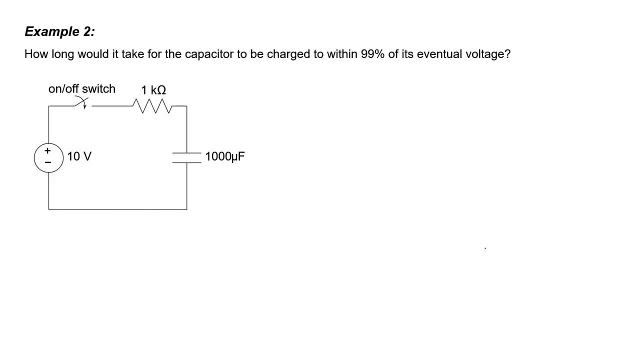 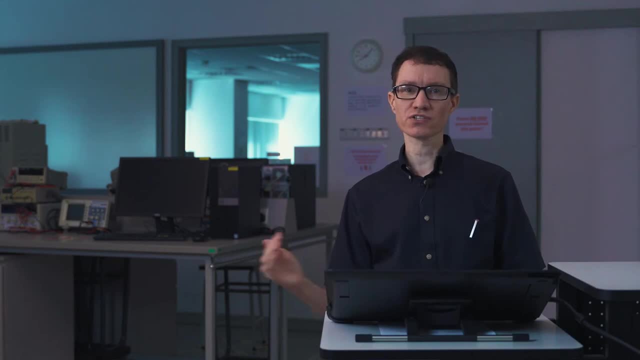 In this example, we're asked how long it would take for a capacitor to be charged up to within 99% of its eventual voltage. We know that as soon as that switch is closed, current is going to start flowing from the source over to the capacitor. 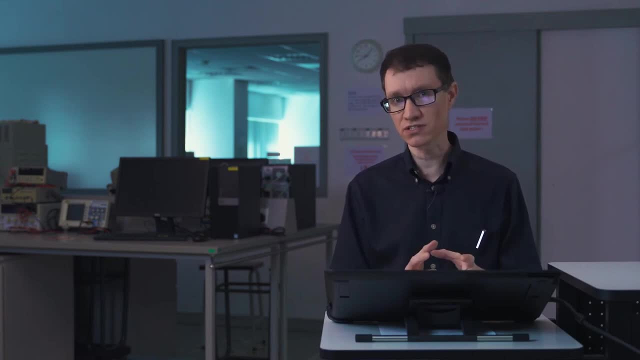 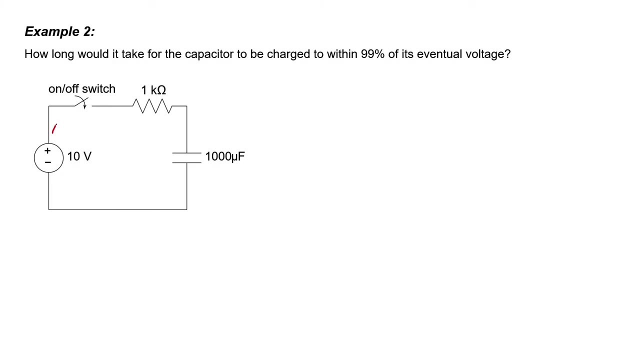 And if we wait long enough, the voltage across that capacitor is going to hit 10 volts. The question here is how much time it takes to get to 9.9 volts. Let's call the current out of that source I. Let's call the voltage here, the DC voltage. 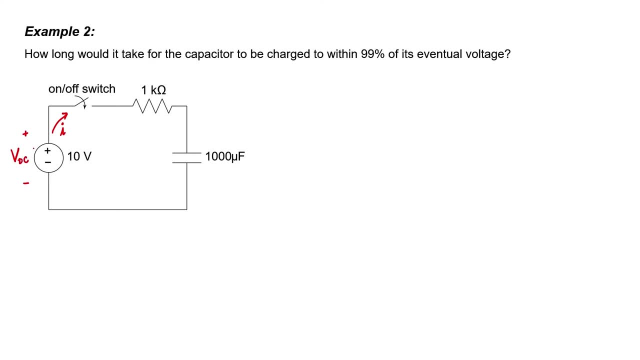 I know it's 10, but I want to keep it in variable form, because it turns out that it doesn't matter whether it's 10 or some other number. And let's call the voltage across the capacitor little v. Let's call this 1 kilohm resistor R. 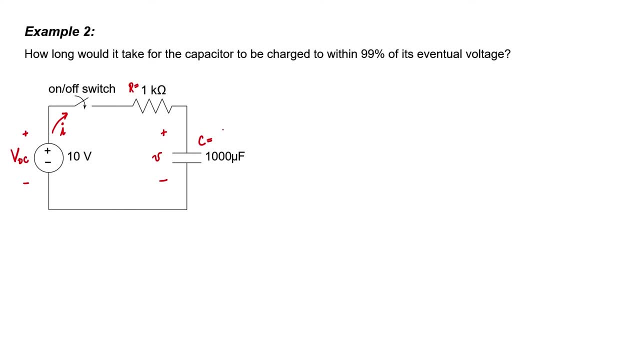 And let's call this 1,000 microfarad capacitor C. I know an equation relating current and voltage in a capacitor. I can also use Ohm's law to relate current and the voltage drop across that resistor. Current is voltage divided by resistance. 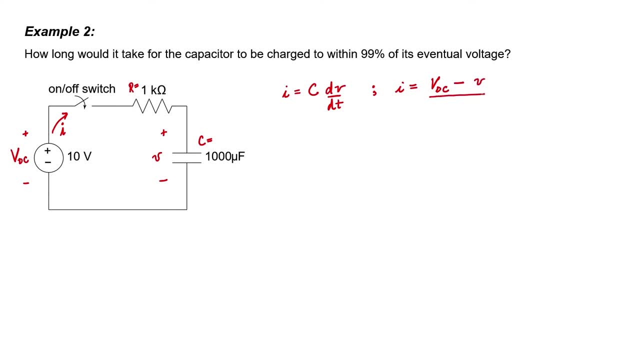 And the voltage. here is the difference from the VDC to the voltage across the capacitor. I can also use Ohm's law to relate current and the voltage across the capacitor. I can set these two equations equal to one another After multiplying both sides of this equation by R. 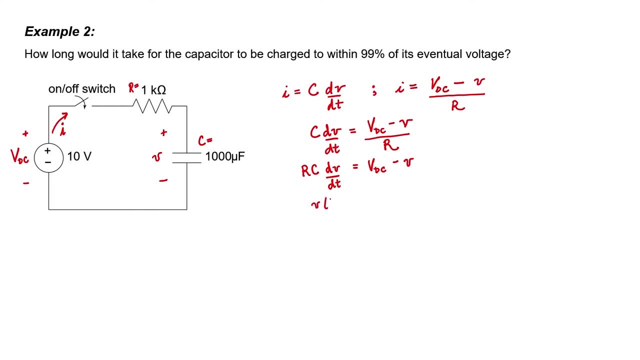 I'm left with a differential equation. I want to solve this equation for V. as a function of time, We've solved this equation in a previous video, so I'm just going to copy down the solution. As you might recall, differential equations in general are not easy to solve. 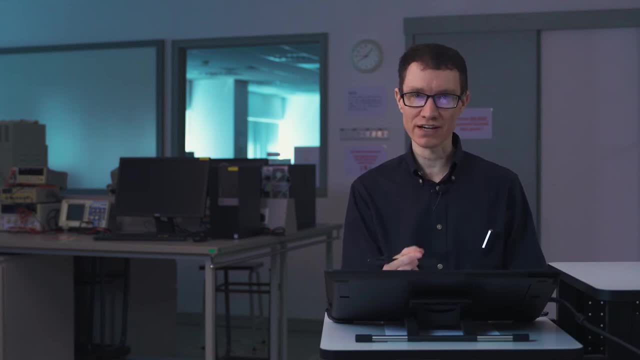 But if you know what the solution is, it's not very difficult to at least verify that this is the correct solution. Since I've done that before, I'm not going to do it now, but I would encourage you to take a look at the previous video. 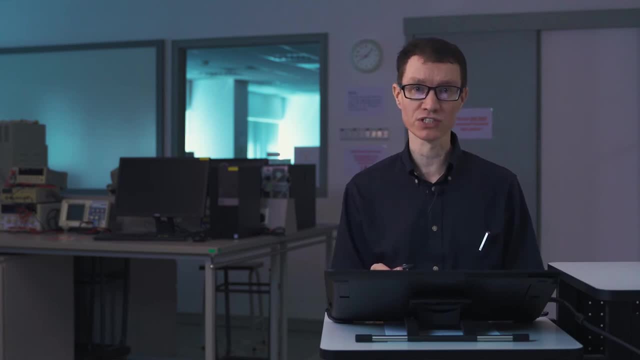 if it's not clear why this is the solution to that particular differential equation. In this problem, I was asked to find out how much time it would take for the capacitor to reach a certain voltage, So I want to solve this equation for T. 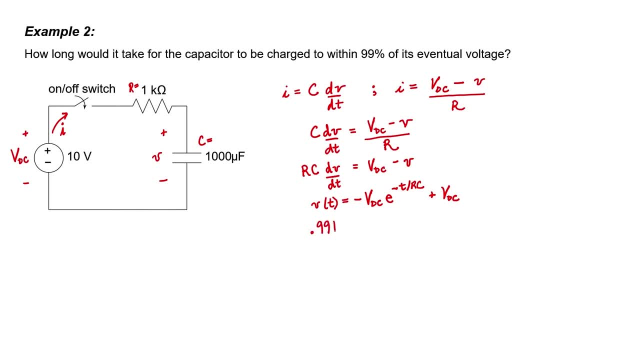 I know that the voltage that I'm targeting here is 0.99 times the DC value, 99% of its eventual steady state voltage. You might notice that the DC voltage cancels out of this equation If I take the natural log of each side. 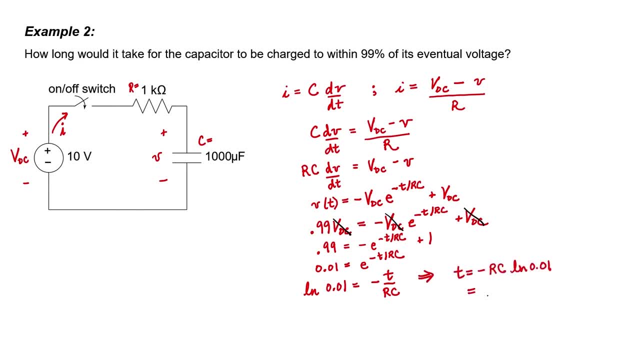 I can get an equation that's easier to solve. for the time, The natural log of 0.01 is a negative number, so I'm left here with a positive time. If I assume that the switch is closed at time, T equals 0,. 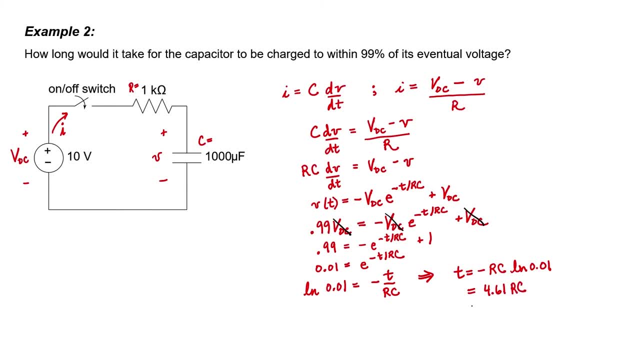 then it's going to take 4.61 RC time constants for that capacitor to reach a voltage of 9.9 volts. In this example, the RC time constant is 9.9 volts, But the RC time constant is 1, or 1 second. 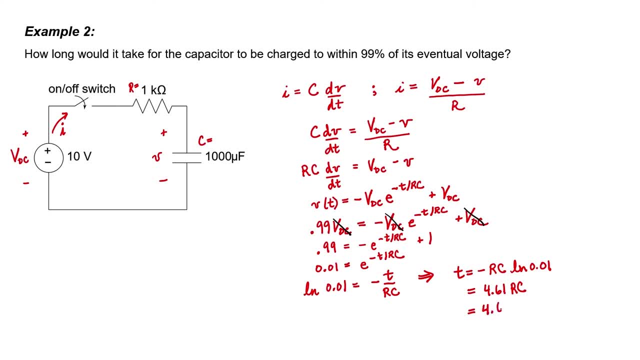 So the time needed to reach a voltage of 9.9 volts would be 4.61 seconds. A good rule of thumb for circuits in general is that it takes about 5 RC time constants for a capacitor to get charged. Strictly speaking, 5 RC time constants. 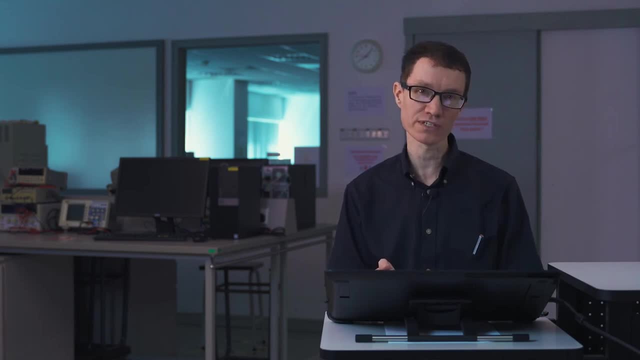 will bring a capacitor up to 99.3% of its eventual voltage, But it's worth remembering that about 5 RC time constants can reach a voltage of 9.9 volts. time constants is what you need in order to get a capacitor charged up In this. 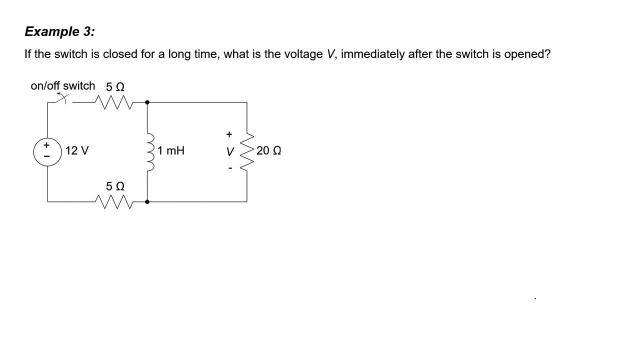 example, we have an inductor and we're told that the switch is closed for a long time and then it's opened. Let's first consider what happens in the circuit when the switch is closed for a long period of time. I'm going to redraw. 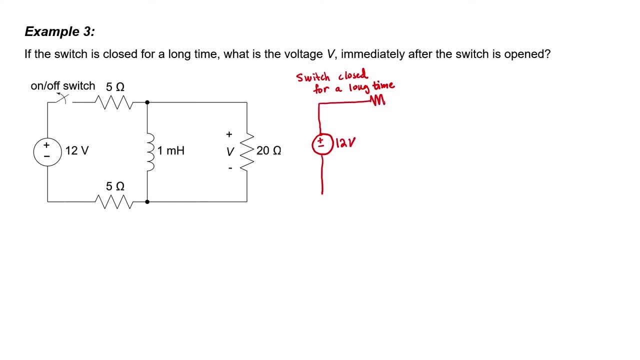 the circuit. to make the situation clear: After a long period of time an inductor behaves like a short circuit. You don't believe me? Look at the equation that relates voltage and current in an inductor. Once the current is not changing anymore, then the voltage approaches zero. I know that after the 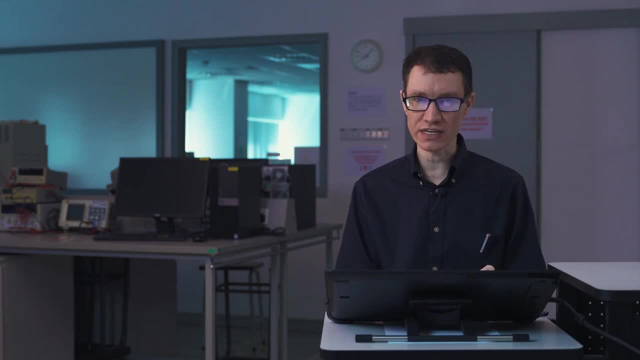 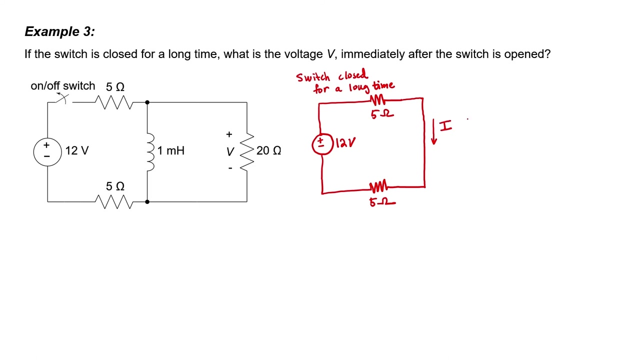 switch has been closed for a long period of time, the voltage V in this circuit is going to be zero and there will be a particular constant amount of current flowing through that inductor. Let's calculate what that current is. I can use Ohm's law, because without the inductor, or with the inductor behaving like a 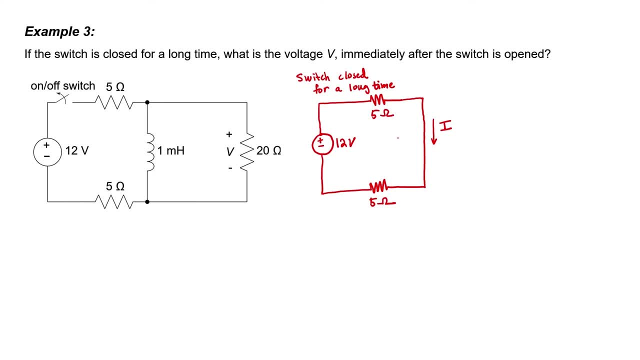 short circuit. I have 10 ohms per second ohms of resistance in this circuit. 12 volts divided by 10 ohms is 1.2 amperes. What happens at the moment that the switch is opened? As soon as the switch is open, it closes off the left part. 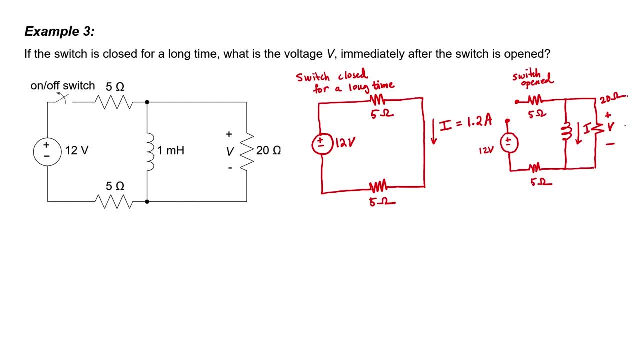 of that circuit completely. There's no current flowing from the 12 volt source anymore, and the only current we have flowing in the circuit at all is the residual current that was flowing through the inductor at the moment the switch was opened. Let's go ahead and erase the part of the circuit. 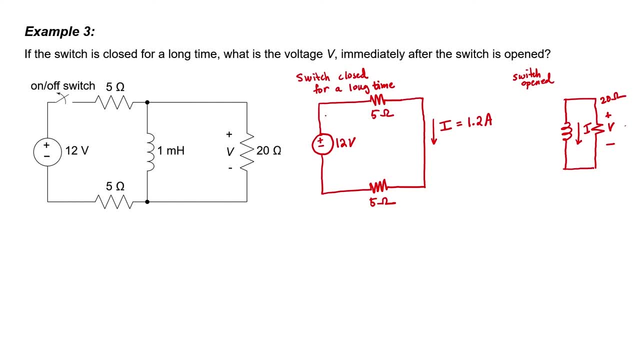 that no longer matters. Initially, after the switch had been closed for a long period of time, we had a particular energy stored in that inductor. You might recall that the stored energy is given by one-half Li squared. That amount of energy is still in the inductor at